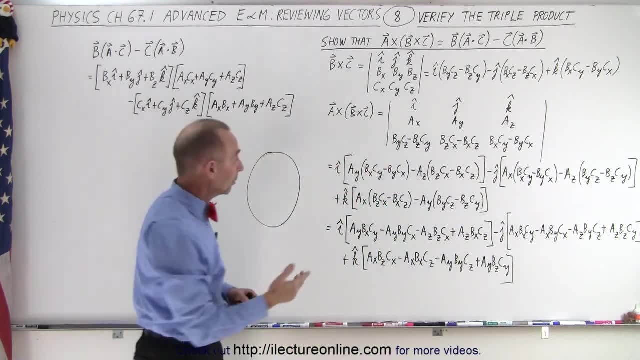 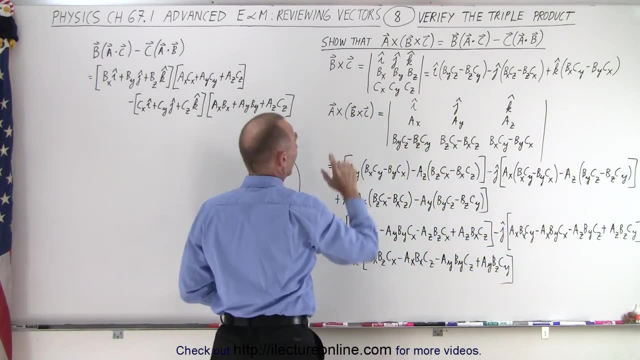 And so when we work all that out, we have this: And then we can multiply the A y times everything inside, the A? z times everything inside, and so forth. So we end up with this as being the left side of that equation: A cross, B cross C. 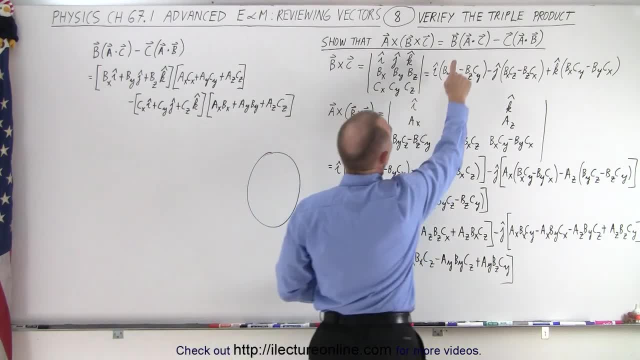 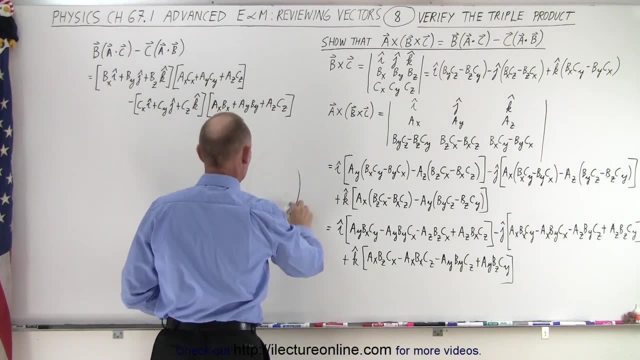 Now we're trying to show That that is equal to B times A dot C, minus C times A dot B, And I still have my circle here that we used to focus on before we started showing the video, So that circle is now gone. 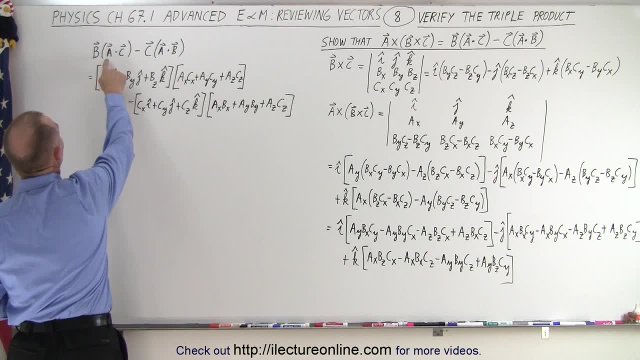 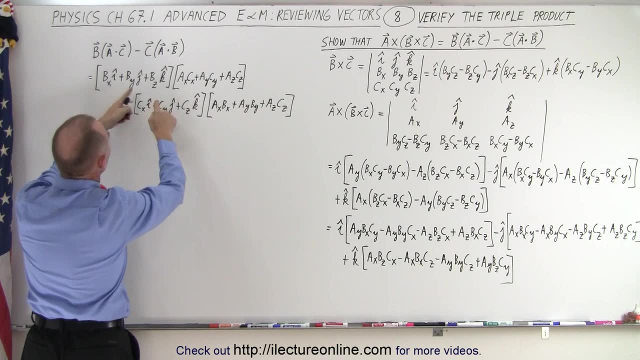 On the left side we started working out B times A dot C minus C times A dot B. So B is simply this vector right here, the B vector, Bx By Bz and the i, j, k components. 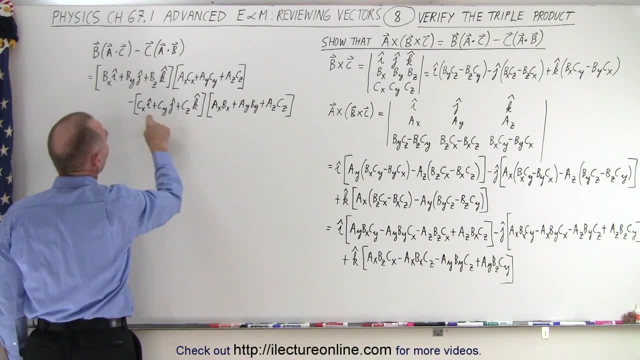 And then C is simply Cx, Cy, Cz and the i, j, k components. Minus is over here. And then A dot C is simply the x components, the y components and the z components multiplied Here. A dot B is the x components, y components and z components multiplied. 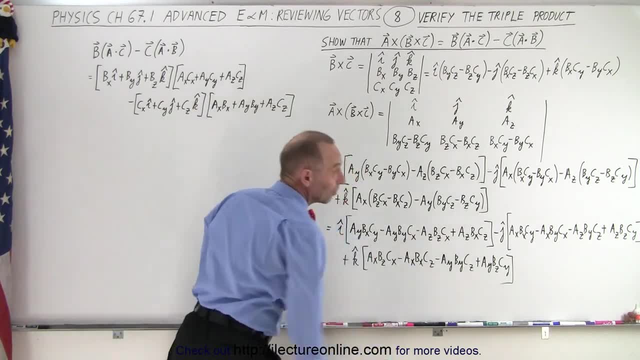 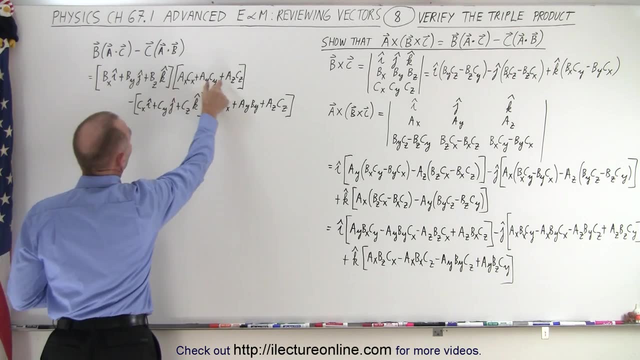 Now, supposedly, this is equal to this. Now let's show you how that's done. So the next what we're going to do is we're going to multiply the Bxi times each of the components in here. So this is equal to, and we have i. 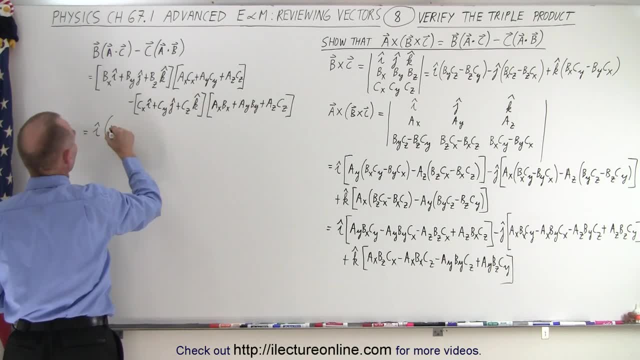 Times Bx, times Ax, Cx. So we have, let's write the Ax first, So Ax, Bx, Cx, Then this times that, So that would be plus Ay, Bx, Cy, And then this component times, this: 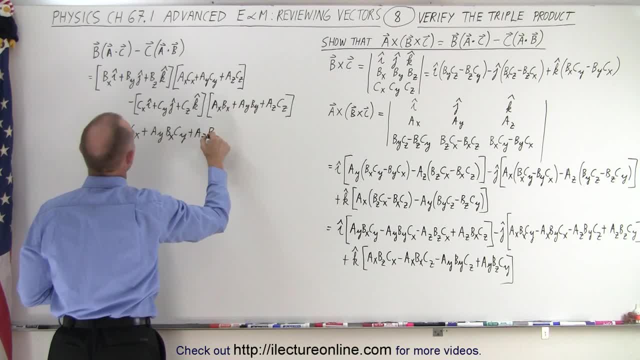 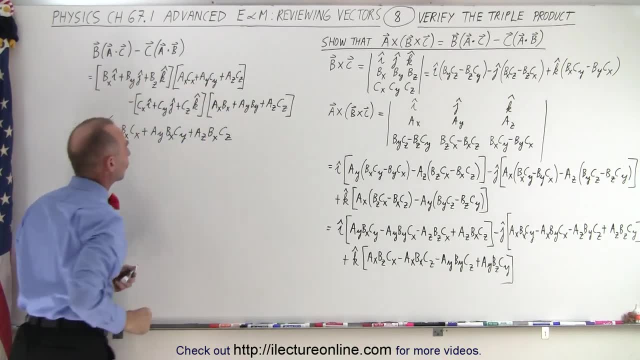 That would be plus Az, Bx, Cz. So all we did is we multiplied this Bxi times these three Terms, right there. And of course I'm going to do the x components first, so the i components first. So now I'm going to multiply this times this. 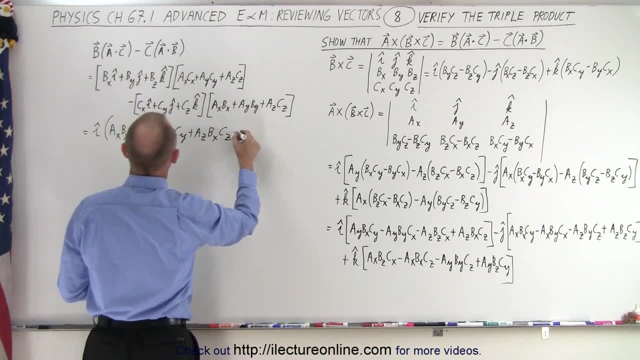 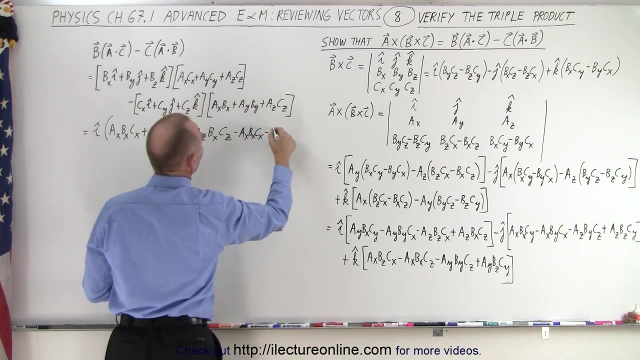 And notice I have a negative here. So that would be minus Cx. Oh, let's write the A first. That would be Ax Bx times Cx. So I'm multiplying this times this And then minus this times this. that gives us Ay By and Cx. 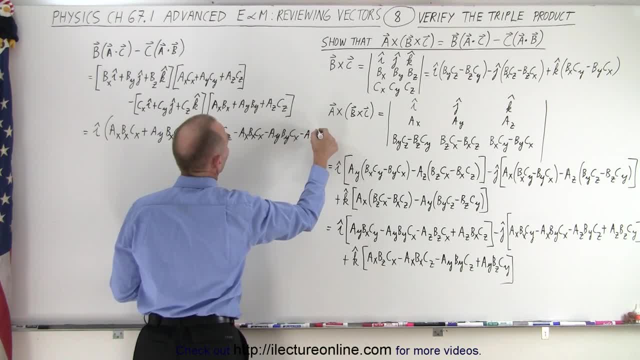 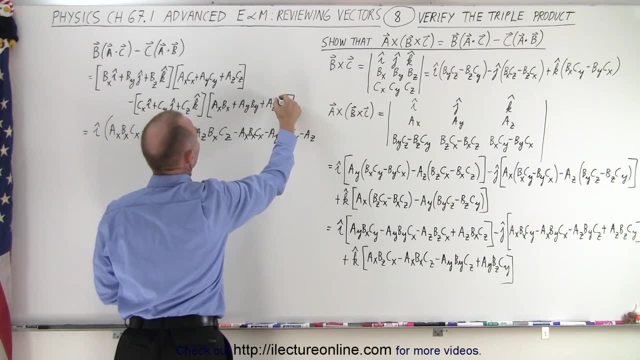 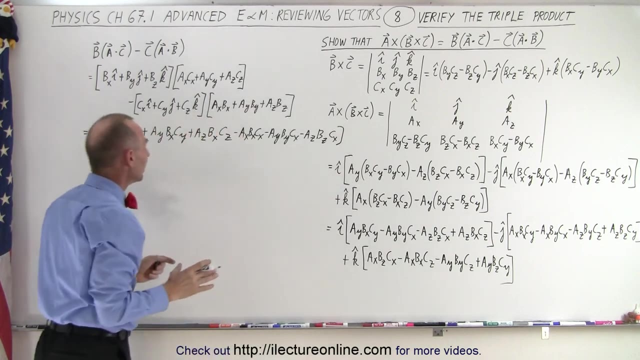 And this times this gives me minus Az. something is wrong here. That should be a B, Bz. There we go, So Az, Bz, and then we have Cx. Notice that's only the i component of the right side of that equation. 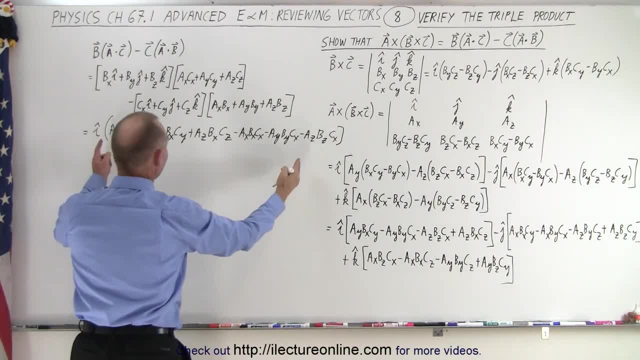 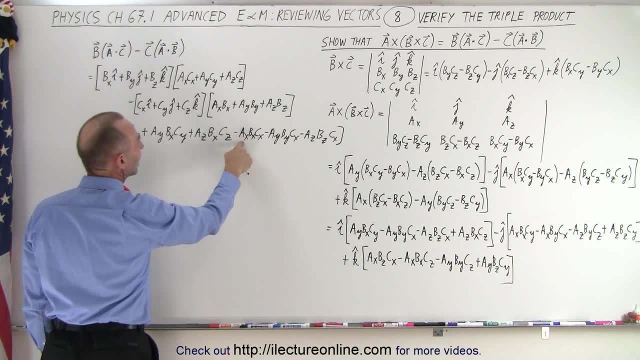 And let's just compare the i component first. So that means that this right here should be the same what we have in here. Now notice, we have an Ax, Ax Bx Cx, Minus Ax- Bx- Cx. 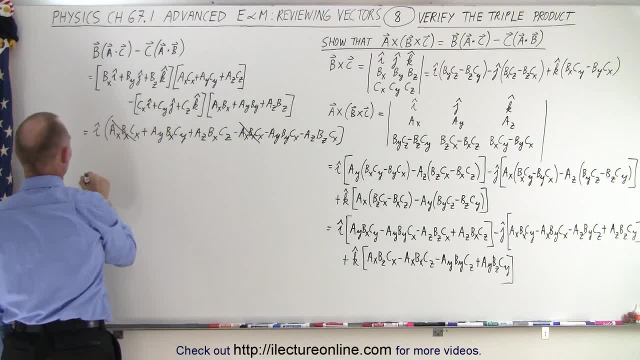 So this cancels out this, And so this is equal to: and let me leave some room for the j and the k components. So for the i component, we now have, we have an Ay, Bx, Cy, We have plus an Az, Bx, Cz. 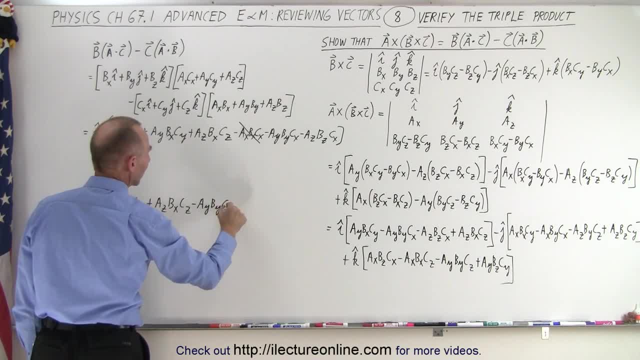 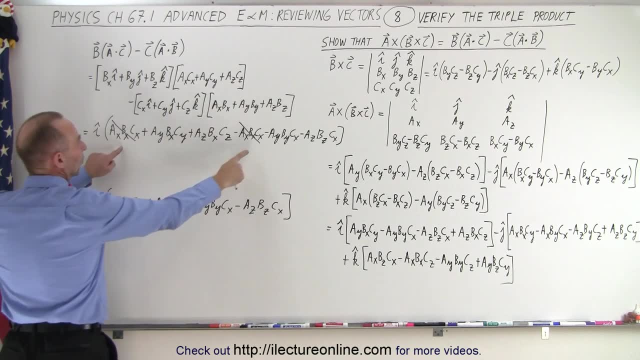 We have a minus Ay By Cx And a minus Az, Bz and Cx. So what I've done is I've simply, once we've cancelled these two out, I recopied the four remaining terms in here. times i: vector. 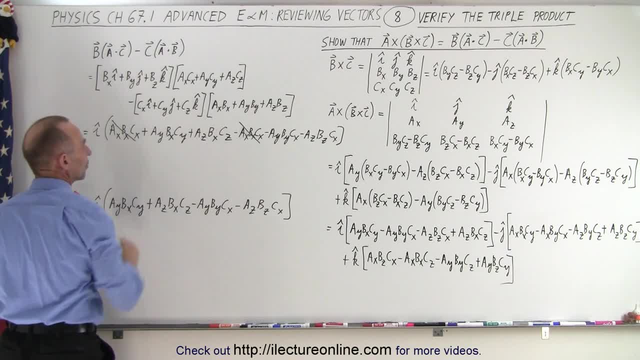 i unit vector, of course, And I can do the same for the j and for the k unit vector, But just let's check the i unit vector alone. And of course I made that a bracket, so let's turn it into brackets. So let's see if we have the same thing. 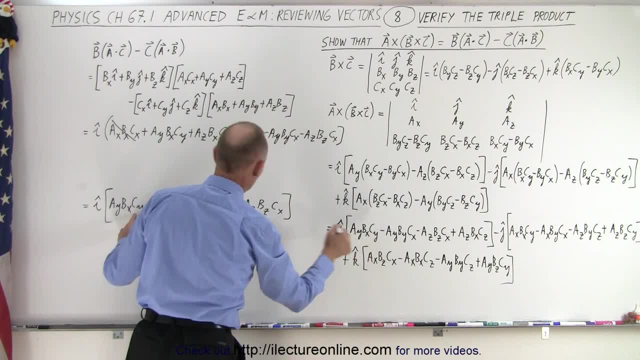 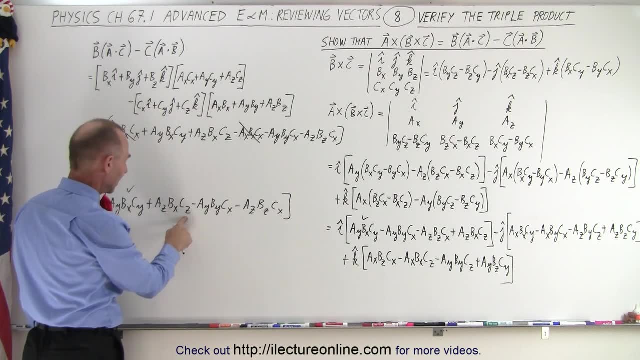 Ay Bx Cy, Ay Bx Cy. So that means that this is equal to this. Alright. next we have an Az Bx Cz. Az Bx Cz. that's this one, right there. 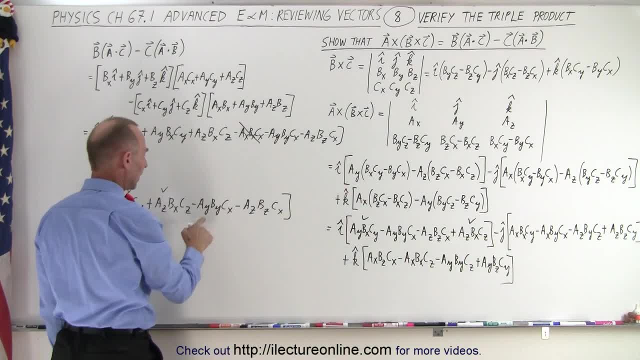 So we have this term and that's this term. How about Ay By Cx with a negative in front of it? Ay By Cx, that's this one, right here, And that's this one, And you have an Az Bz Cx. 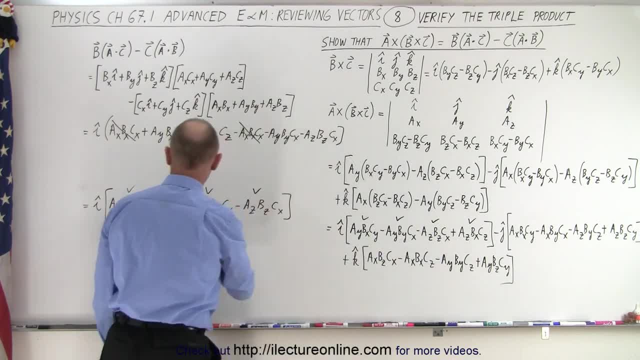 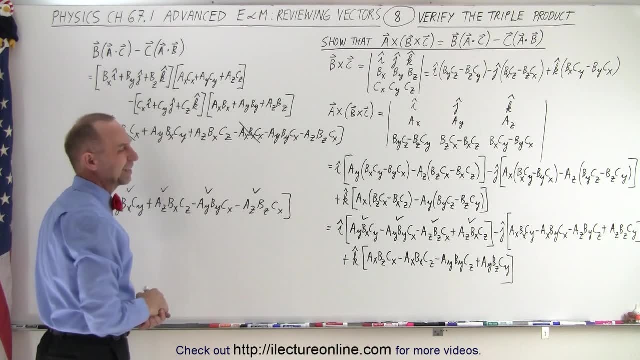 Az, Bz, Cx with a minus. And notice, we found all four terms over here. We found them over there. At least that showed that the i component was the same. Let's do it for one more component, the j component, to see if we have that correct. 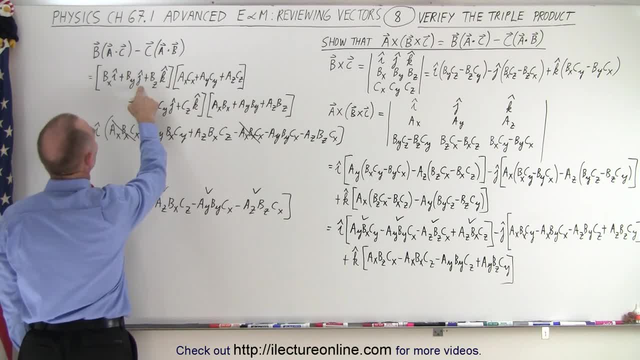 So let's see, here We have a j component right here And we have a j component right here with a negative. So plus j times By times this. So we have By times. oh, I want to write the A first. 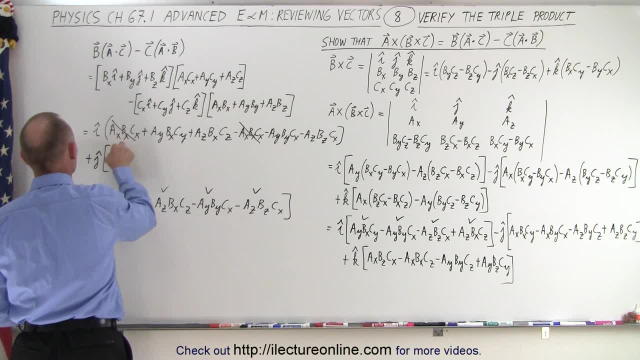 Because if we keep it in the right order that makes it a lot easier to work with. So we have this, times this. So we have Ax By Cx, And then plus Ay By Cy, plus Az By Cz. 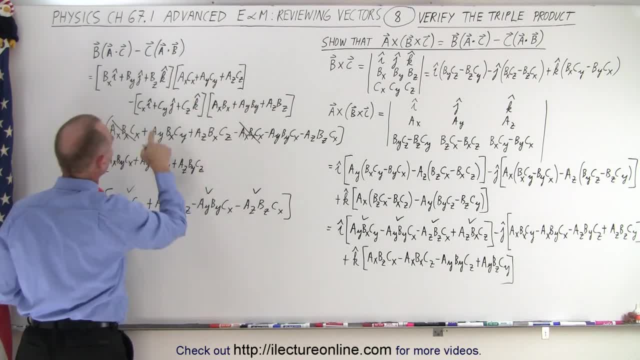 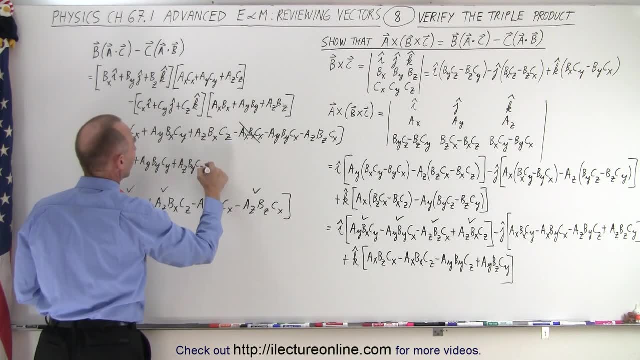 So we multiply this times, this. Now we're going to add these terms together. So here we have the Cy in the j direction, but in the negative. So we have Ax, So minus because we have a minus here, So minus Ax, Bx, Cy. 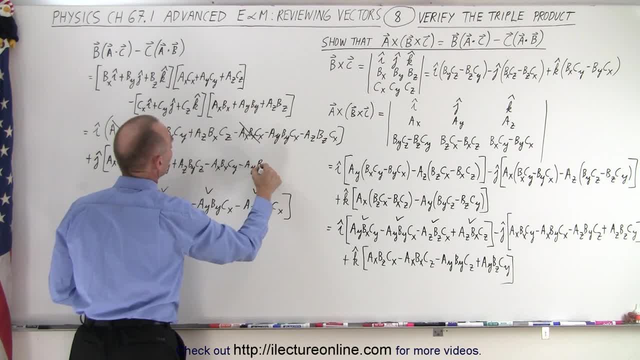 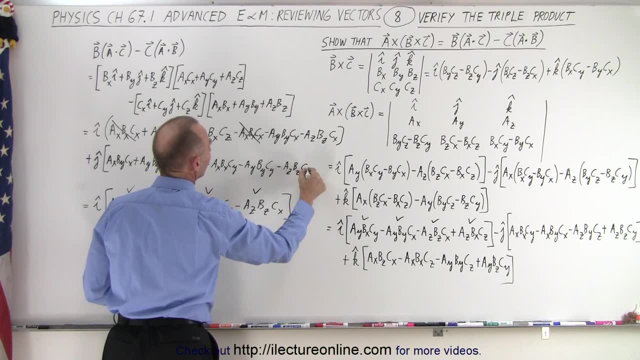 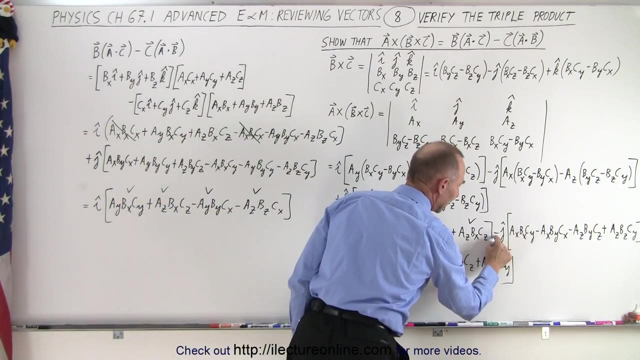 And we have a minus Ay, By and Cy And we have a minus Az, Bz and Cy. Okay, so that's the j component And that should match our j component over here. Now be careful, we have a negative sign here. 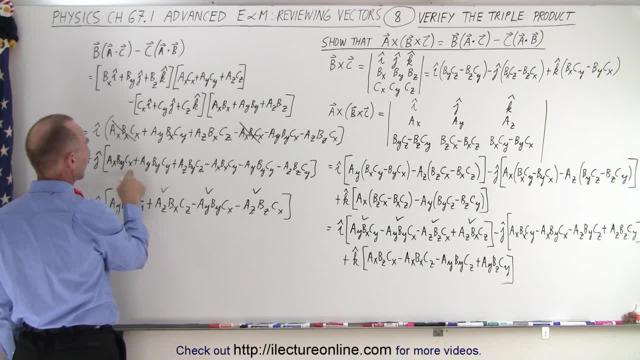 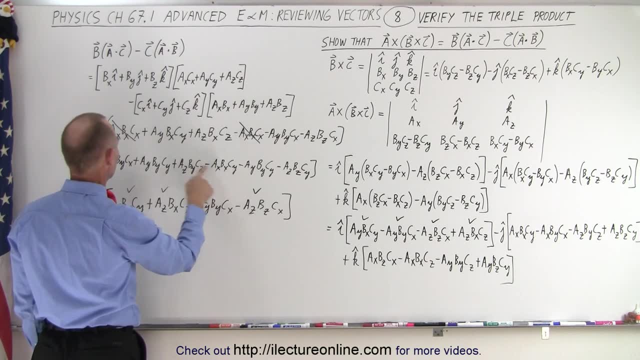 And we have a positive sign here. Also, we have an Ax By Cx, Ax Bx Cy. That's not the same. Let's see here: Ay By Cy, Ay By Cy. So this cancels out with that. 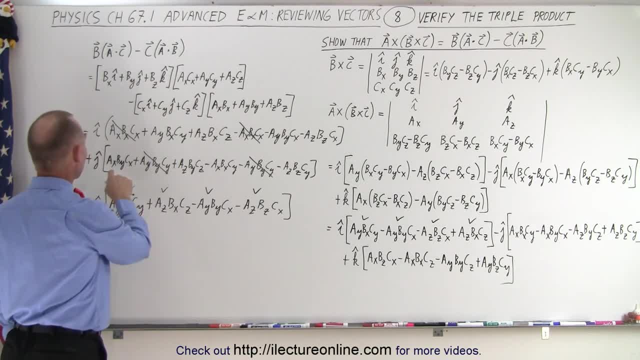 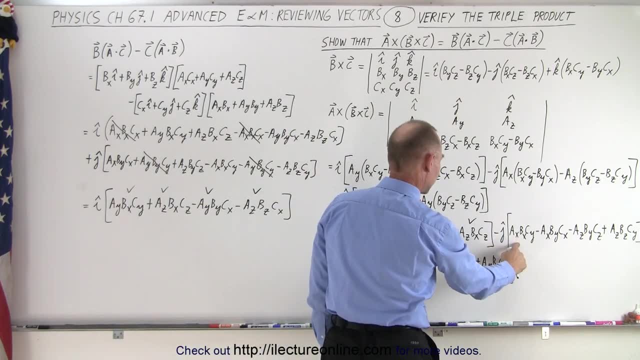 That makes it a little bit easier. Now let's see if we find the four components that are the same: Ax By Cx. So we have. where are we here? Ax, Ax, So X, Y, X, X, Y X. 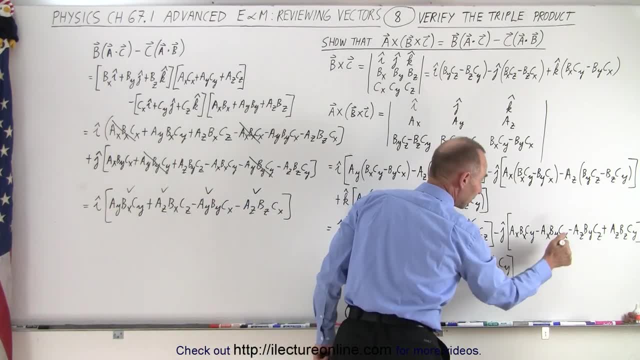 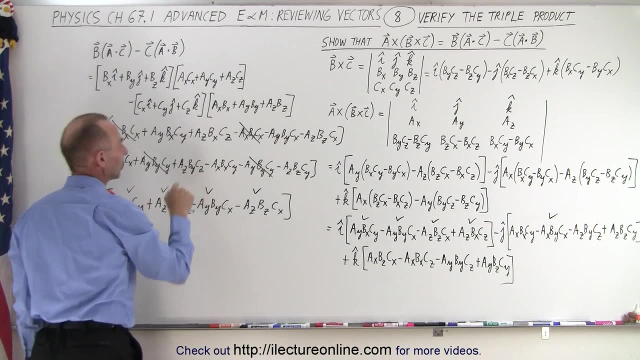 I have a positive here, I have a negative here, But this negative makes that positive, So this one is the same as this one right here. So we have Az. So Z Y Z, Z Y Z. I have a negative times. a negative is positive. 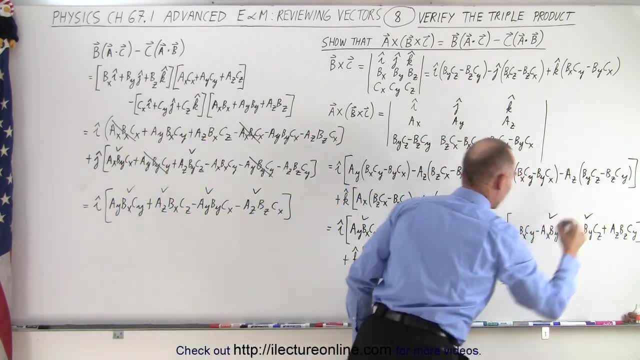 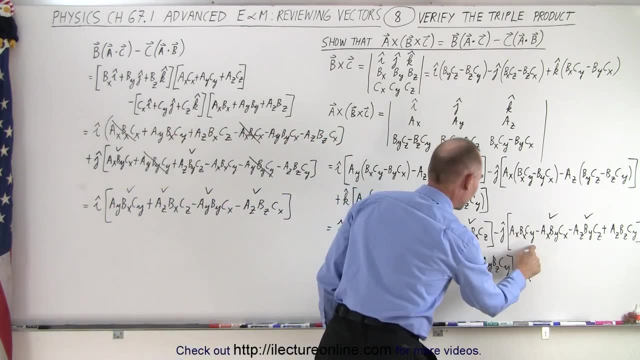 And I have a positive here, So this matches this one right here. And let's see what else we got. We got a minus. Ax, Bx, Cy, X, X, Y. I have a minus, I have a minus. 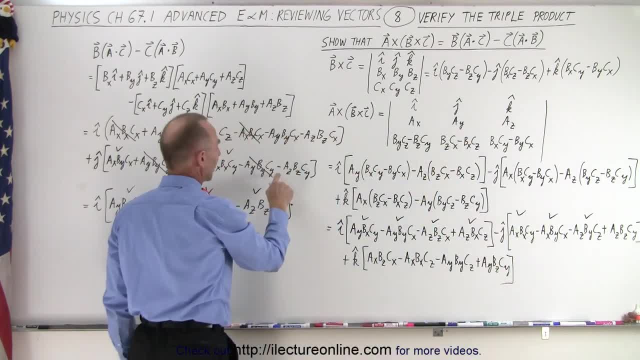 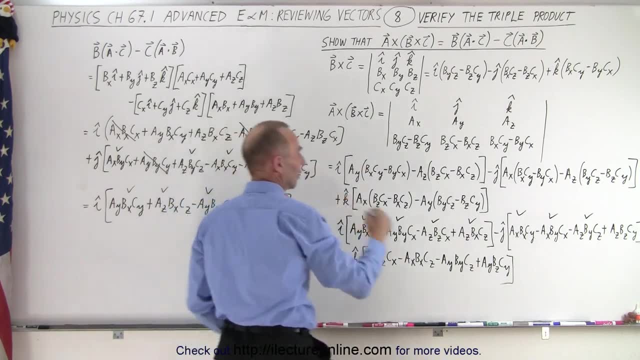 So this matches this one right here, And I have a minus: Z Z Y, Z Z Y. This plus with this minus makes that a minus, That's a minus. So this matches this, And so I've shown you that at least the I component is the same. 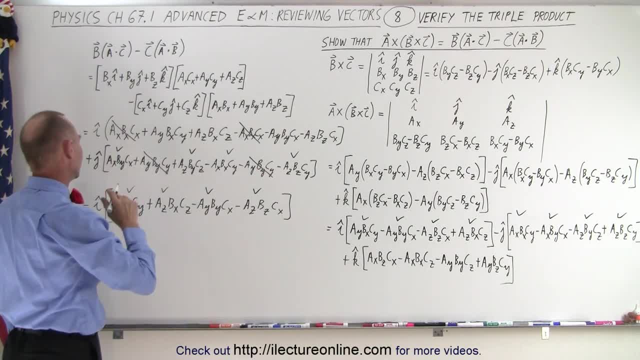 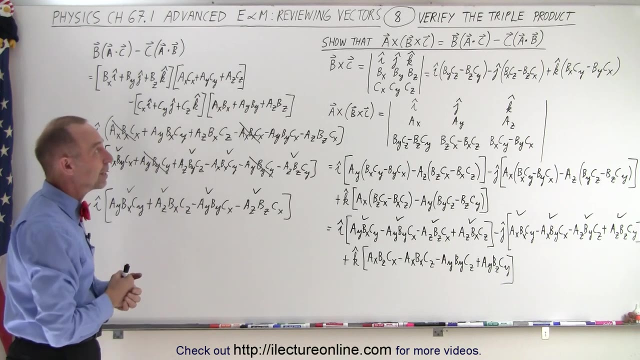 The J component is the same And since I'm running out of room, we can assume the Z component is the same. Well, anyway, that is how we show that A cross B cross C is the same as the back cap: the B times A dot C minus C times A dot B. 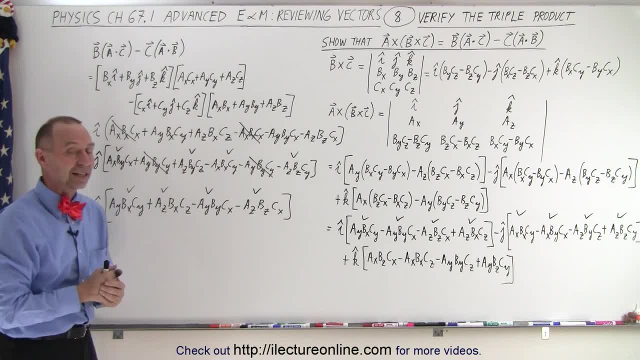 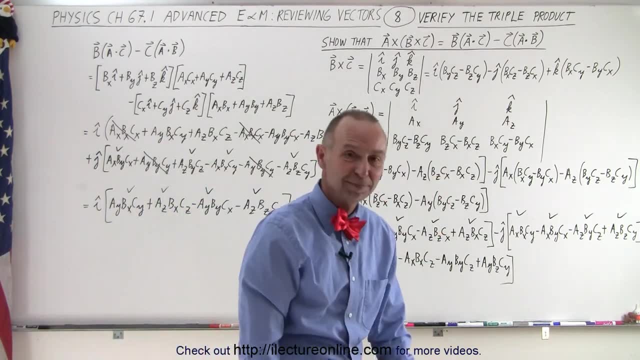 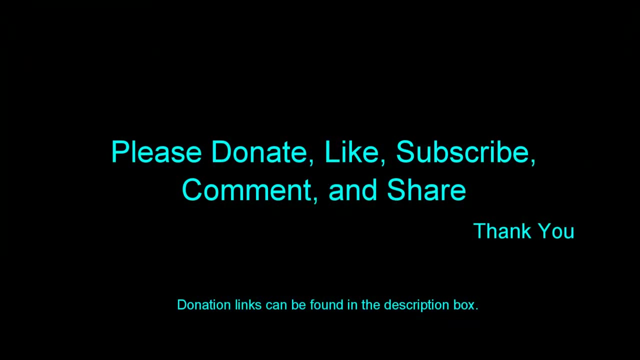 We verified the triple product. that is exactly the same thing And that is how it's done. 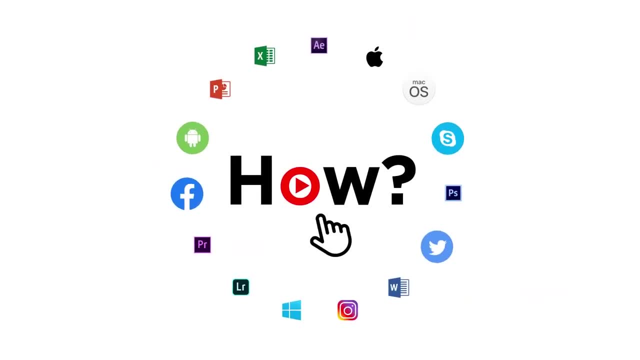 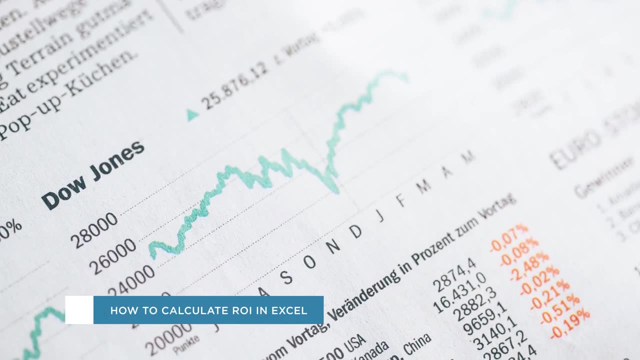 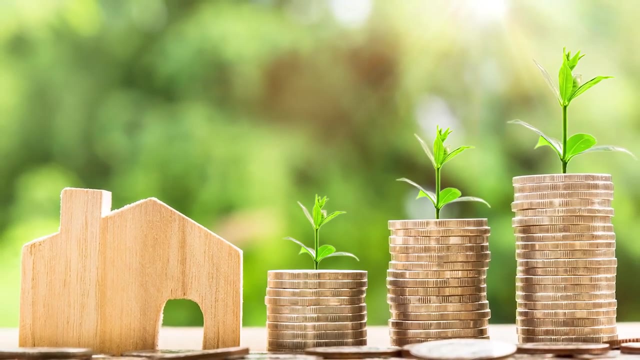 Hey everyone, welcome to another Howtech video tutorial. In this video we'll be showing you how to calculate ROI- return on investment in Excel. ROI is a popular metric used to determine how good an investment is by comparing the initial value of the investment with the final value and getting